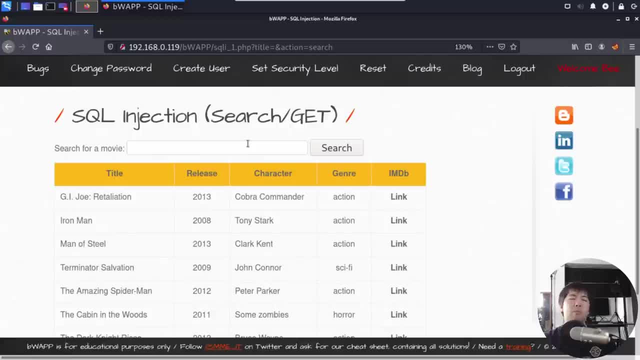 query: is it vulnerable to SQL injection so that we can run all of our attacks following from there? And that's the key part, actually, because if you are able to find a vulnerability, that will be much easier for you to pull out all those information like usernames and password. 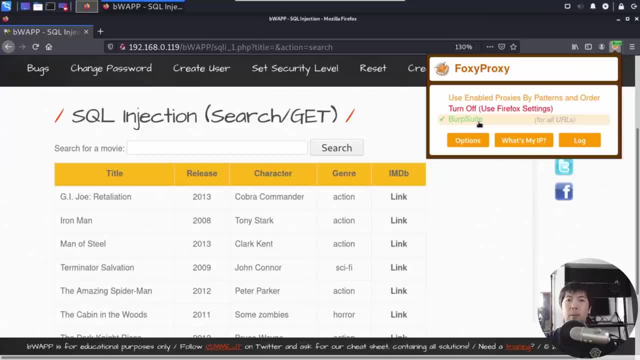 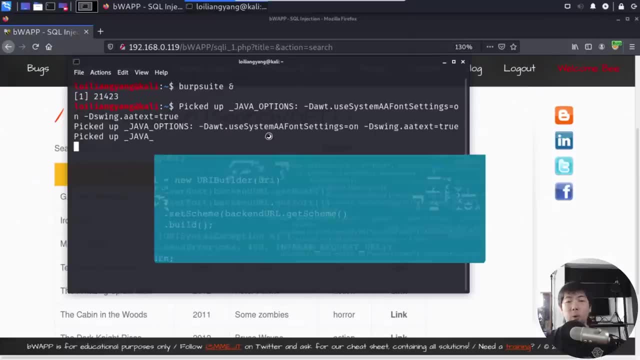 view. So what we can do is go to the top right corner, select Foxy proxy, select burp suite, And go ahead and open up terminal. All right, so what we can do now is go ahead and launch burp suite from here, And we have, of course, the burp suite community edition. So let's go ahead and launch. 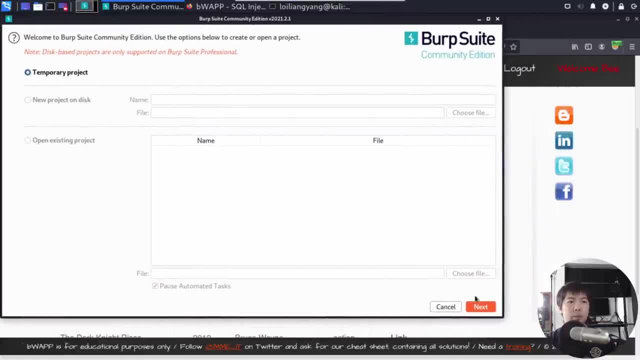 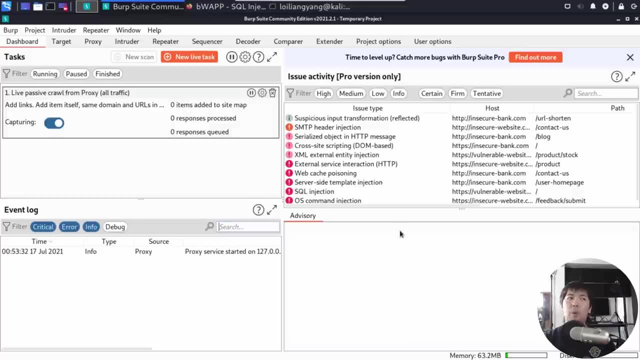 just that. So here we have the community edition, And what we can do now is click next, click start burp, And this will begin starting burp suite. So burp suite is going to be our interceptor, So it will intercept all the requests that we're sending over into the site, And once we send it over, we 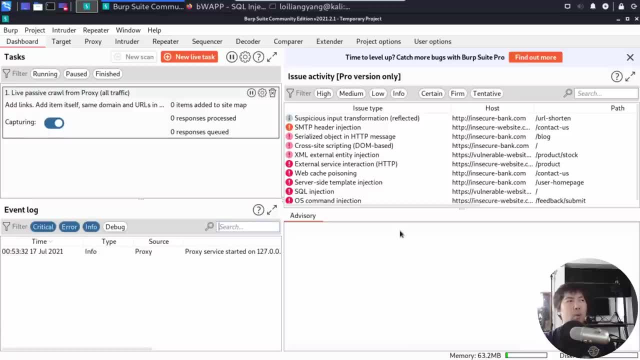 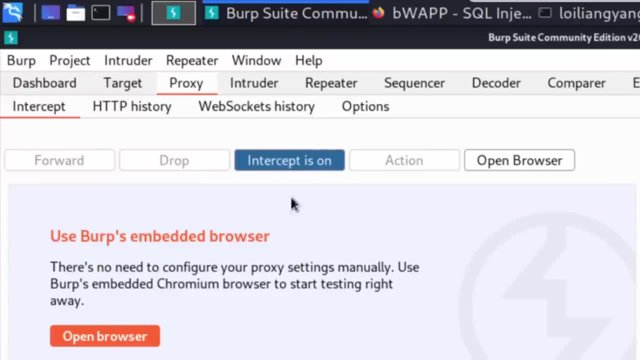 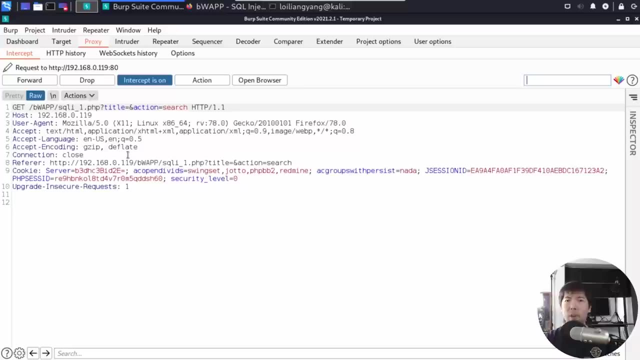 can change up the data. we can change up the information and see whether the particular field is vulnerable to cyber attacks. Okay, So we can go under the proxy tab, ensure the intercept is on. go back to your browser, All right, click search again And there it is. we have the interception right here. very, very simple. 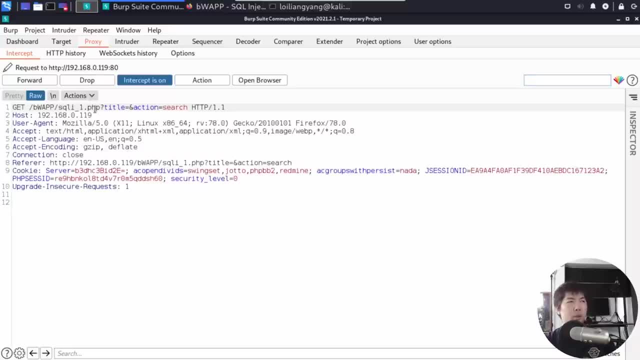 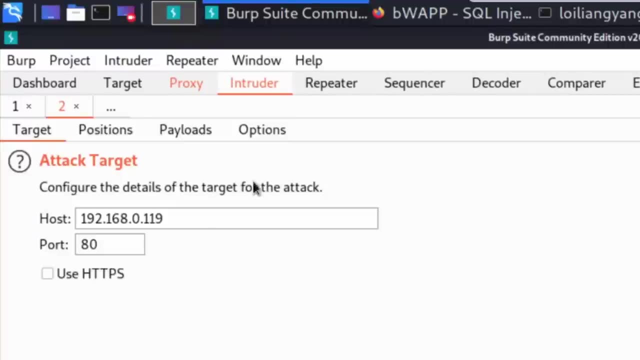 way of being able to change up those data. So what we can do now is do a right click and send over to intruder. Okay, so once you're under the intruder tab, here we have the attack target. So this is. 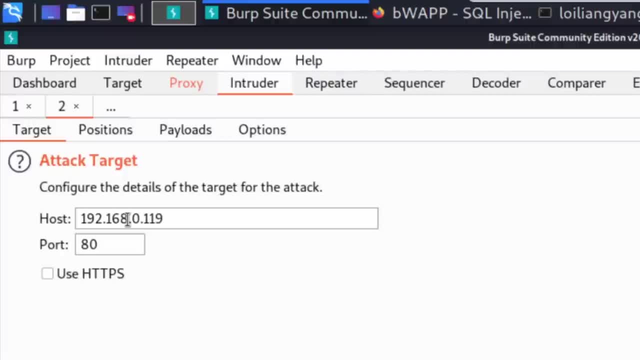 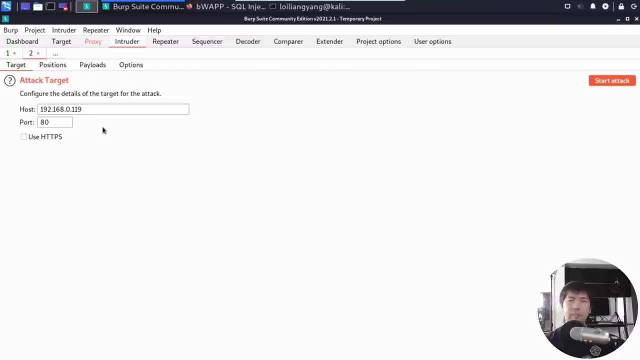 the host name And in our case, we're running in our own virtualized environment. So in this case, in this situation, we have the host IP address And, of course, in the real world you're targeting a specific domain name, All right, And at the bottom you have: 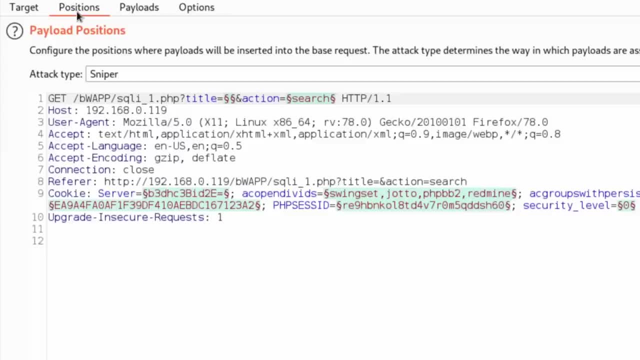 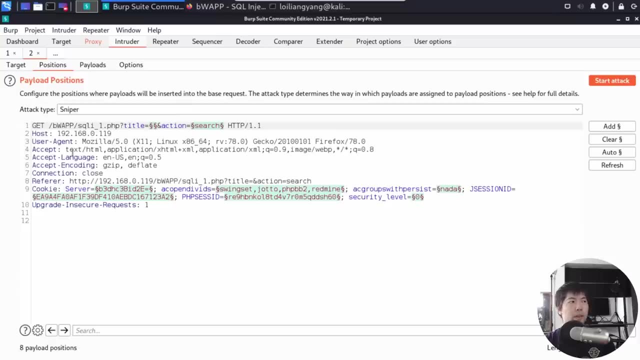 the port number. in this case we're port 80. All right, And of course, we have positions, And this is a really important part to understand. okay, regarding positions. So here we have the haters. we have haters like host, user agent, accept, accept language, accept encoding And you may. 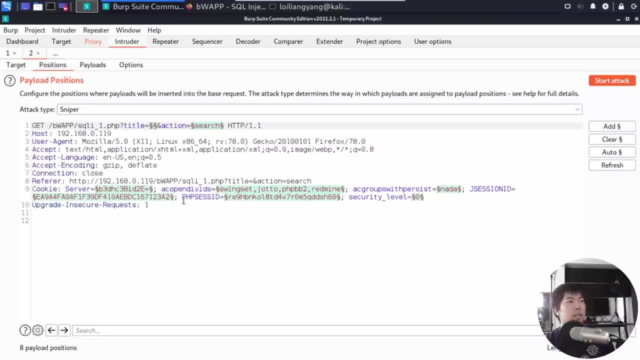 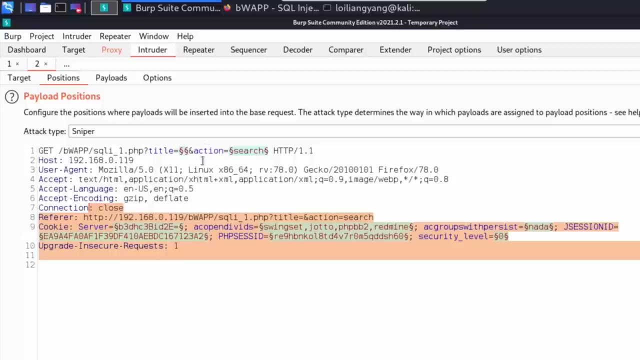 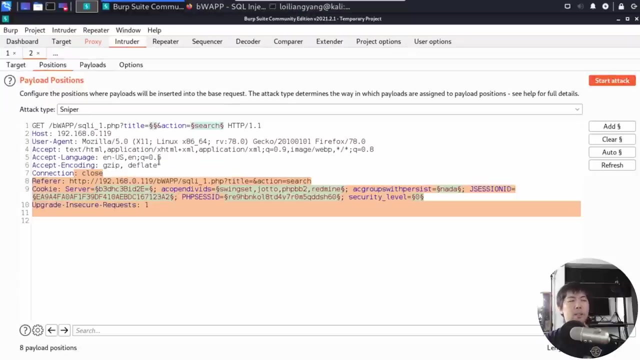 sometimes tend to overlook some of this very, very important information inside the haters And there are many situations in which, okay, this is an injection point. it's not just in the Get slash, BW APP SQL underscore. i dot php title. So we are going to target title as the place for us to launch a SQL injection. However, many of these haters could be also sent over into, like a database system or data processing for analytics, And once it is being sent over, they can be targeted as well, Because those checks, those input, may not be sanitized. So it's not just the title. 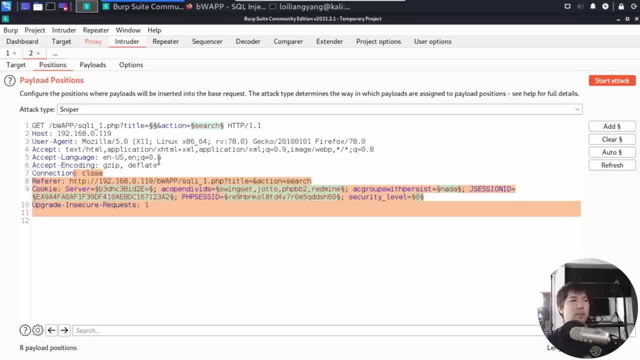 all the usual places that we inject into as the place or the opening for us to check on the vulnerabilities. so now i can go to the right side and click clear, okay, and at the top we have title and action. so i'm going to clear for the action. okay, so we are using an action equals search. 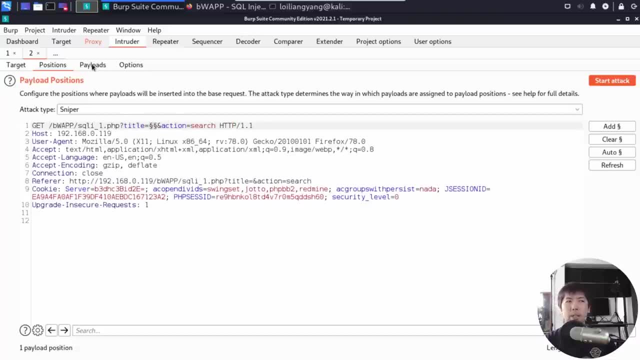 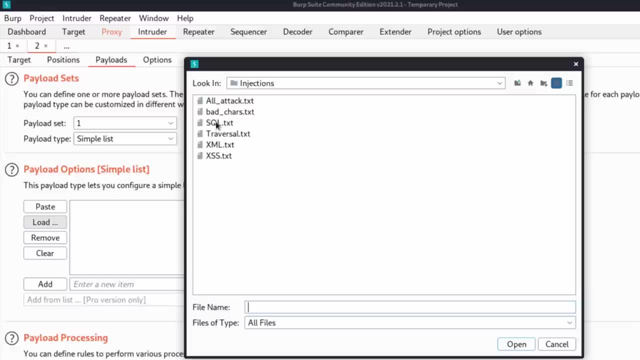 and here we have the title view. so what i can do now is go ahead and click under payloads and in this case i can load up one of the common, all right, sql structured query language injection payload. double clicked on it and see: right here, okay, we have the payload options, all right. so 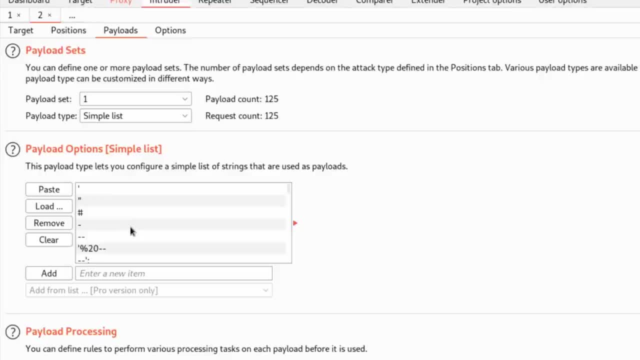 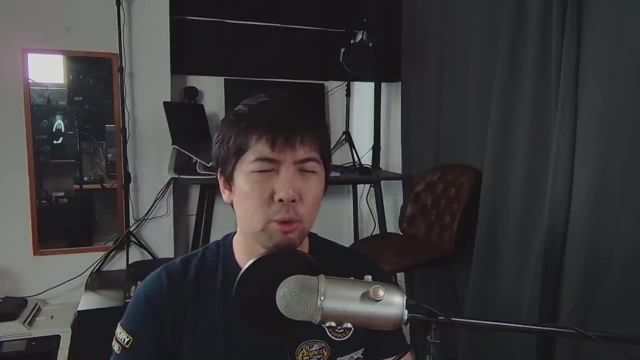 this is a simple list, so we have single code, double code, hex, dash, double dash and a huge list of them, and in the real world, when you're doing a bug bounty check, you're going through tens of thousands of payloads. all right, rather than a simple list like this, because you have 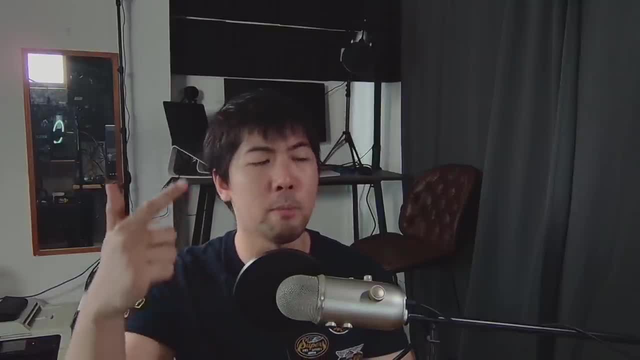 to craft them yourself. you have to use different kind of advanced techniques to bypass those checks. they are done either at the web application firewall level or at the application level, or at the application level or at the application level layer doing sanitization checks. so you want to think about how those applications are deployed. 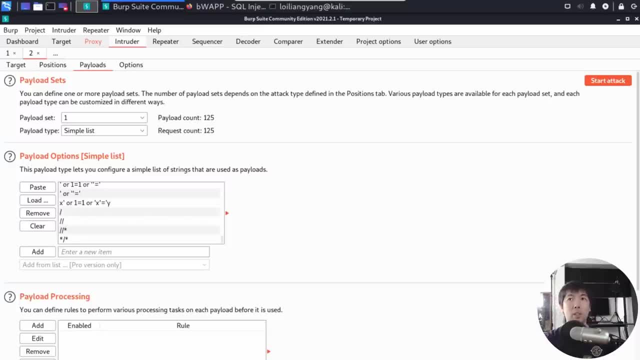 in the real world and then launching attacks against those application systems. so this is really critical to understand. so, going back into burp suite, we can go ahead and click start attack in three, two, one start attack, all right, click okay. and here it is okay, we have the intruder attack one. 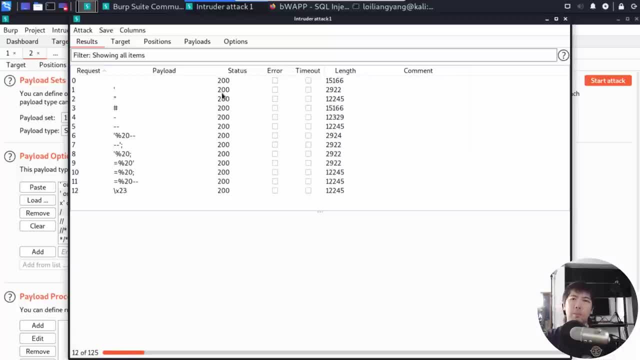 and we have the status, and what we are looking out for is a specific type of error, all right- or looking at a specific way the application server is interacting with our sql injection payload. so now i can click on to say one of them here, and in this case we have the request. 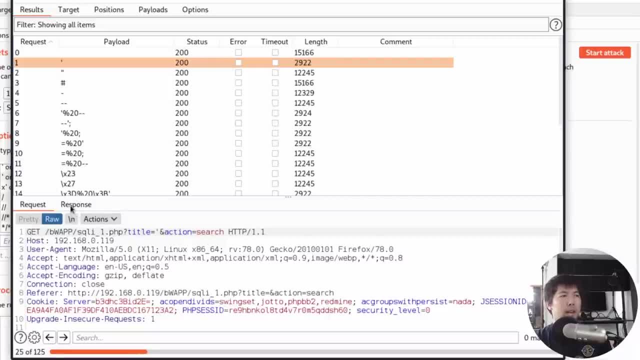 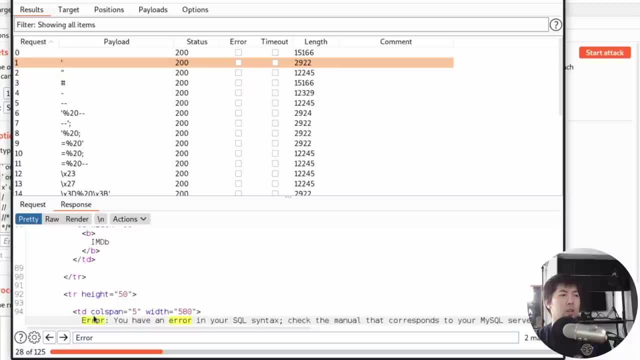 and the response. all right, as you can see the bottom of the intruder attack and if i click on the response here, okay, so as you can see right here we can enter, say, for example, error. so you can see, here we have. you have an error in your sql syntax and you can understand directly from. 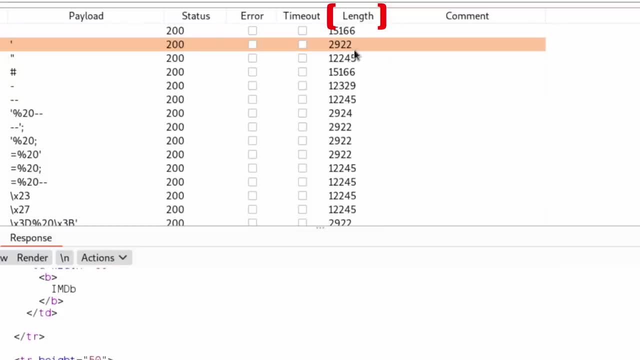 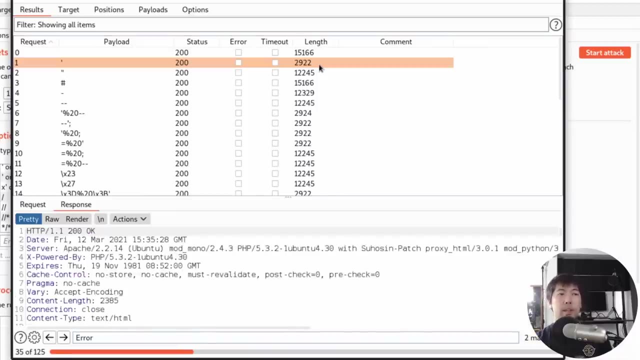 here which one is working and which one is not. so here we have the length. all right, so the length can be one telltale sign that the payload is working. all right. so we have a single quote and there's an error if i scroll down further. all right, i go to the second payload. 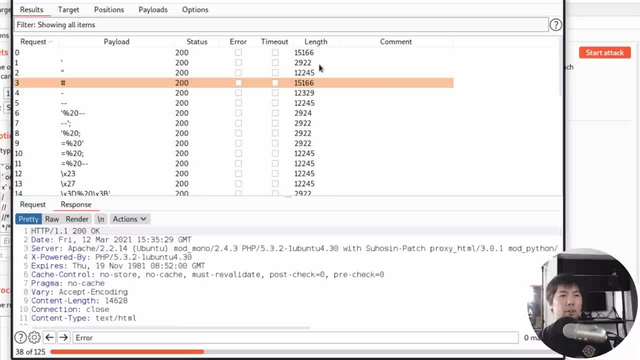 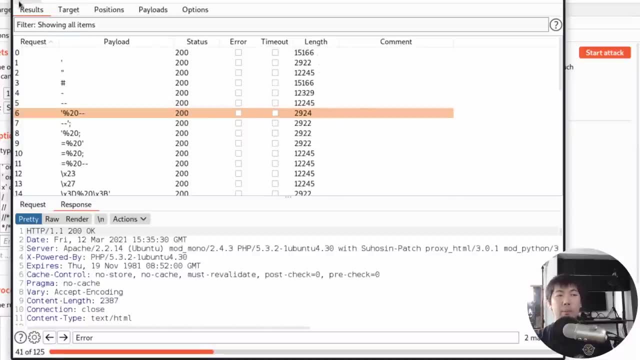 here we have a double quote. it's not working, and you can see from the length here. all right, once again it's not working. but if i go to another one which has a single quote followed by a percent 20 with a double dash, this won't work. all right, as you can see, here we have the error in the search. 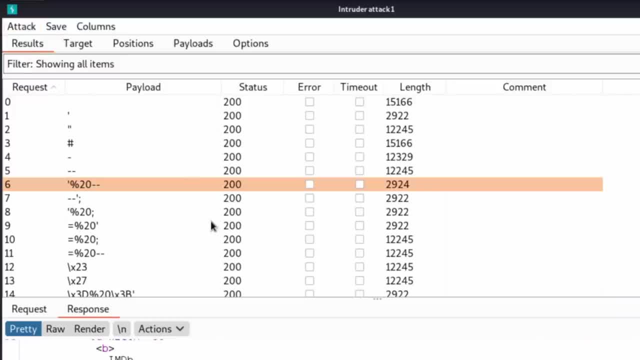 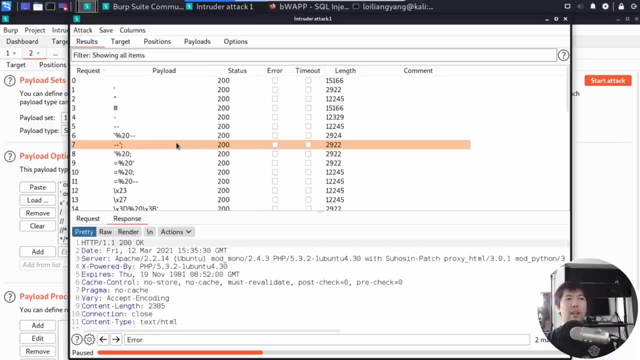 from the sql syntax and what i'll do now is go ahead and pause, all right, the attack. so, as you can see, from the results of all of our sql injection payload, we're seeing that the length, that is, 2922, seems to correspond to the cyber attack or the payload and indicate that it is. 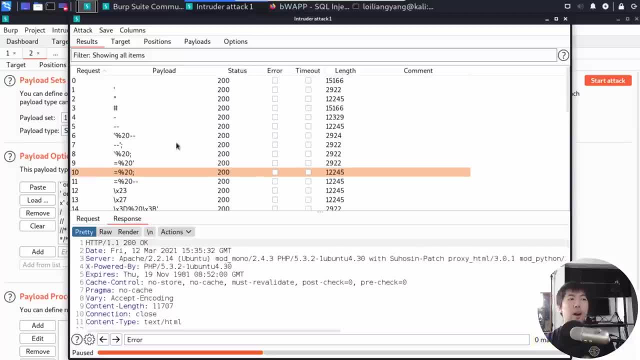 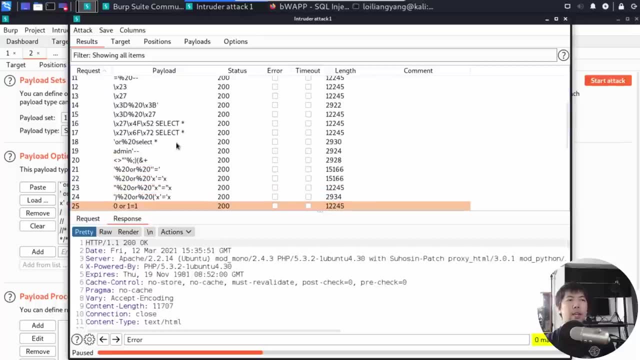 working. we are getting error messages and, of course, those without the single code. you realize that it is not working. okay, so the whole idea. then the question is: is there any way for us to test further to know whether the attack is actually working or not? okay, so if i go back, 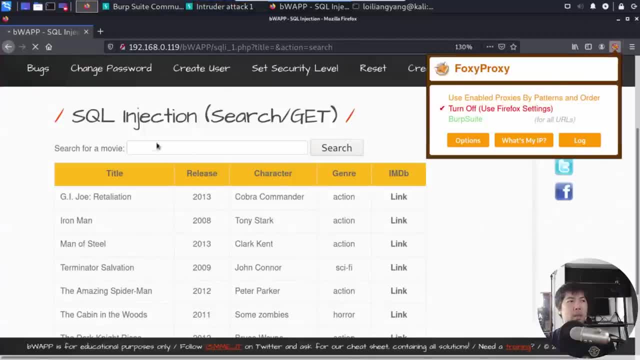 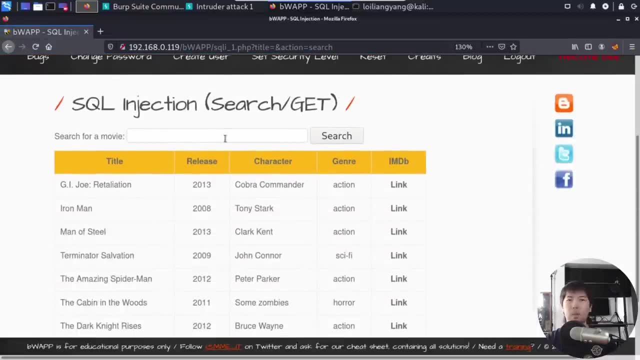 into the browser. all right, and i turn off burp suite for now, and what i'll do is go ahead and stop loading of the site. i click search again. okay, so we are able to see that. okay, we are getting back the common information from the rows and columns. and now, if i put a single quote and i click search, 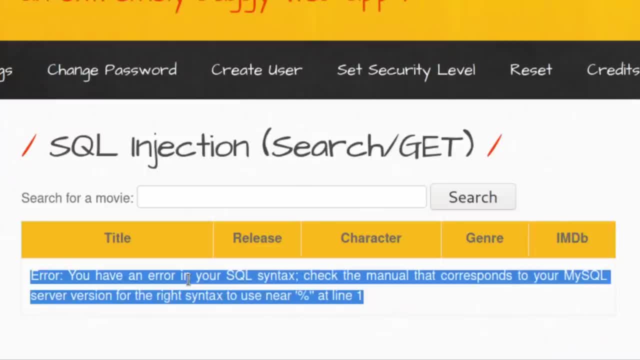 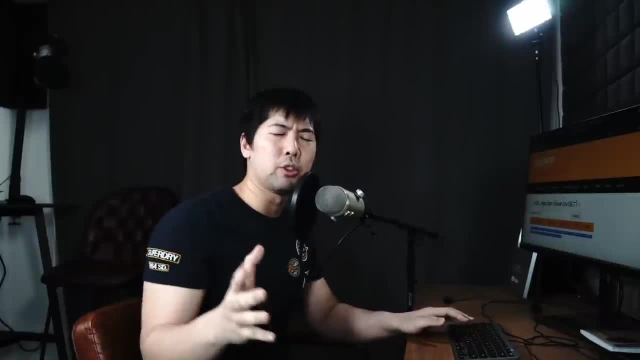 all right. if i scroll down further, you can see over here error. you have an error in your sql syntax, so this is an indicator that a sql injection payload went through. so now the next question you'll be asking is: does this work in the real world? and i want to tell you the idea. 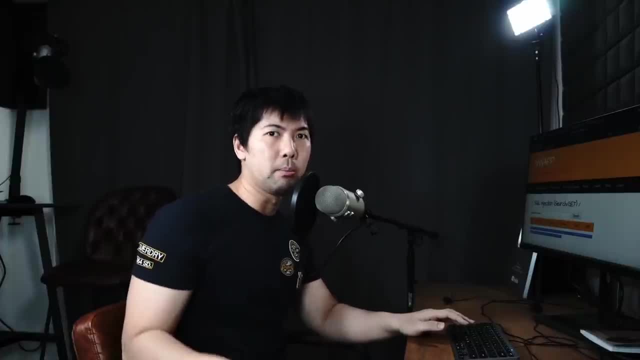 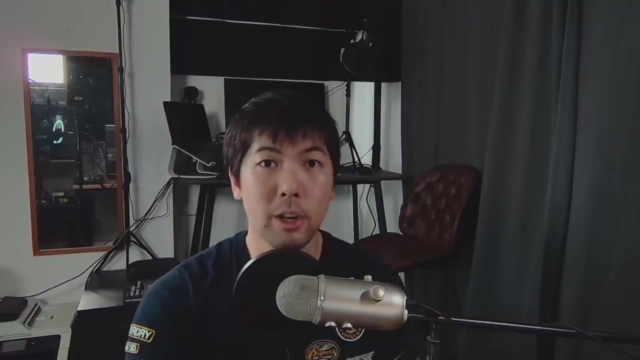 is that? yes, it still does work in the real world, but it's not that simple because there are a lot of sanitization check and web applications firewall. there are a lot of sanitization check and the application layer. the next question is: what advanced techniques can we deploy as part? 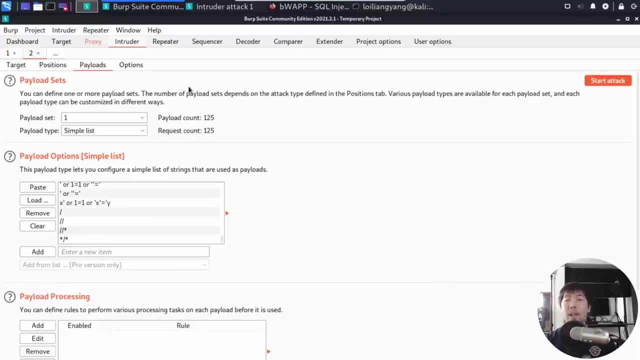 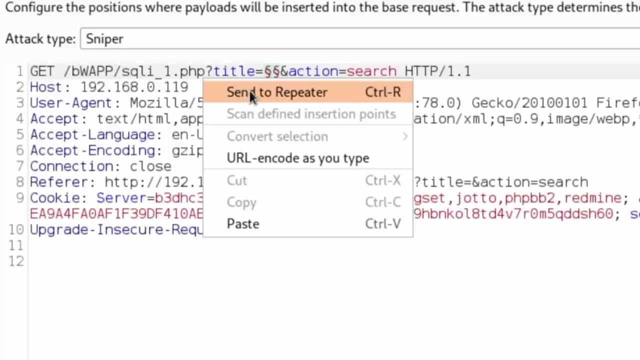 of the attack. well, going back here under burp suite, one of those advanced techniques that you can actually use, i'll go back to intruder. okay, i can click under positions and i can do a right click and can send over to repeater. once i send over to repeater here, as you can see, we have the 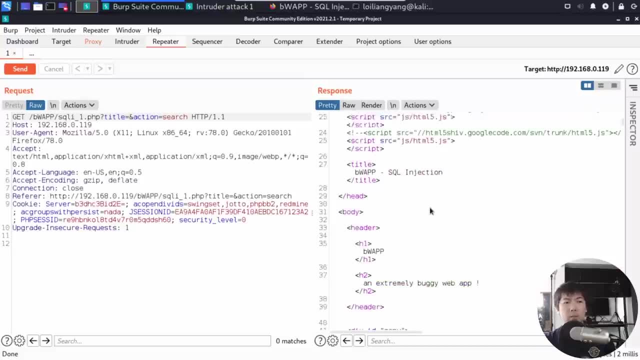 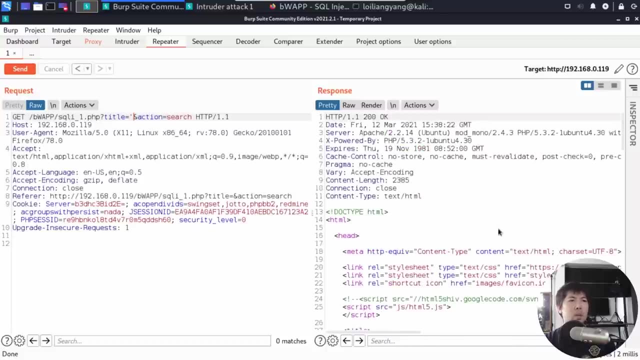 following. so if i was to go ahead and click on the repeater and i can send over to repeater and i can click send, we get a response to the right side, all right, so we can see all the response of all those titles and so on. and of course, if i do a single code and i click send, what if it doesn't? 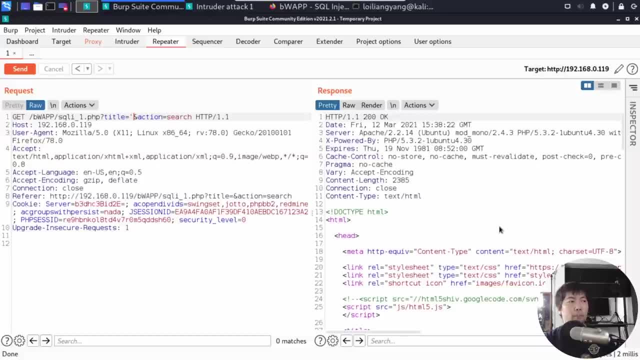 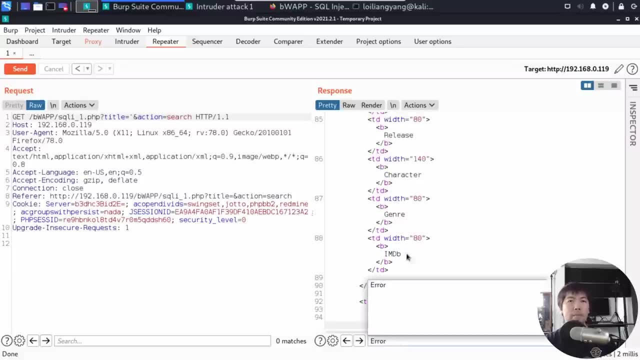 work. okay. let's say in the real world there's some kind of sanitization check before the payload is sent over to the application server. so obviously it would not work. there would not be an error all right inside the response. okay, so in this case one better we can use is go under the decoder tab. 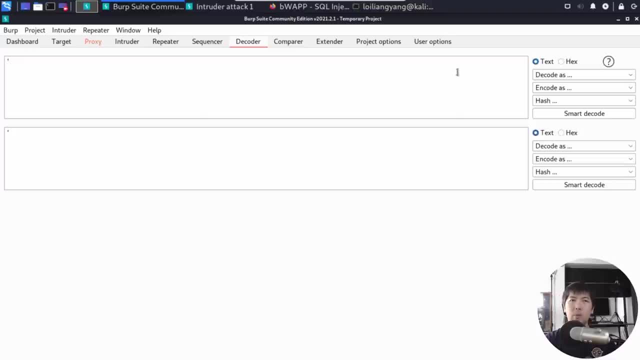 and in decoder i can put a single code, and what i can do now on the right side is to look at the following, which is encode as url. so here in case, say, for example, the web application firewall, the application server, they're looking out for some kind of special. 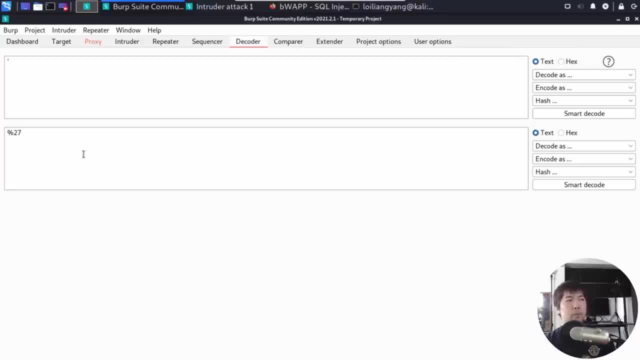 characters that are injected into the web application server in those parameters, in this case, all right, it will not be able to detect a single quote, all right, so here, if i copy the following: so, which is percentage 27? i copy this, i go back into our repeater tab and i'll change. 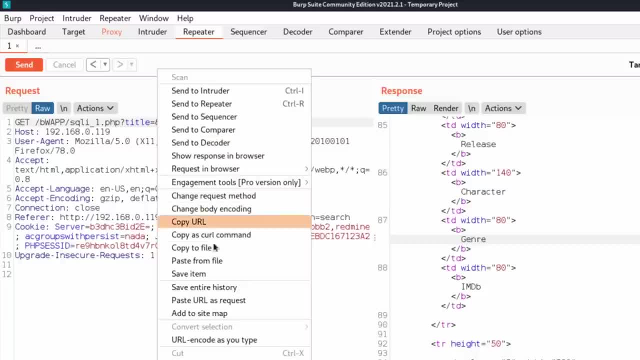 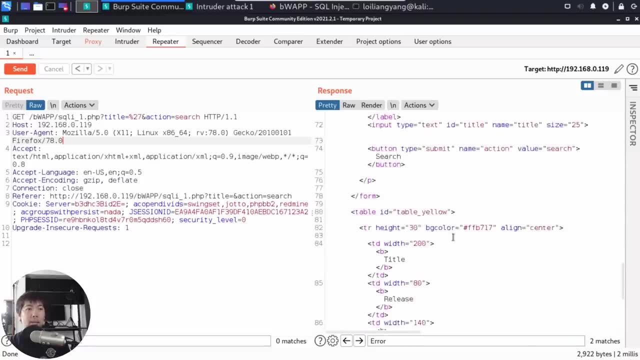 this over and i can do a right click and i can paste it right here. all right, i'll paste it right here so you can see here we have percent 27 and when i click send and as you can see here, i still get error messages. all right, so you can see at the bottom error you. 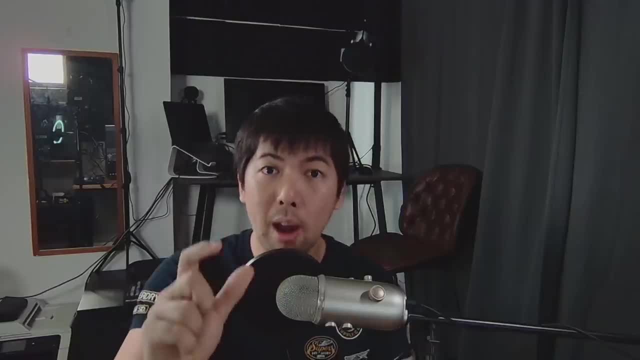 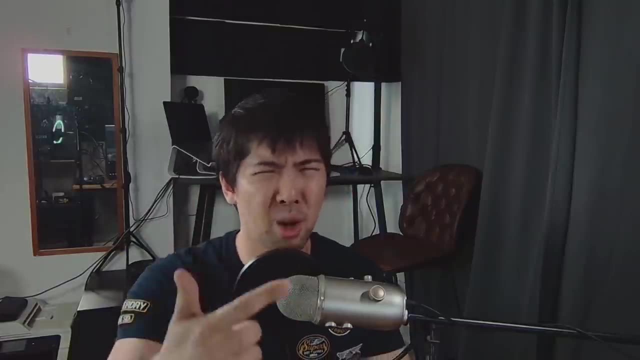 have an error in your sql syntax. so in this case we're trying to look out for vulnerability into different input fields that we can try to bypass, so we can be using encoding, double encoding, and there's a huge list of all these advanced techniques that we can deploy to find those. 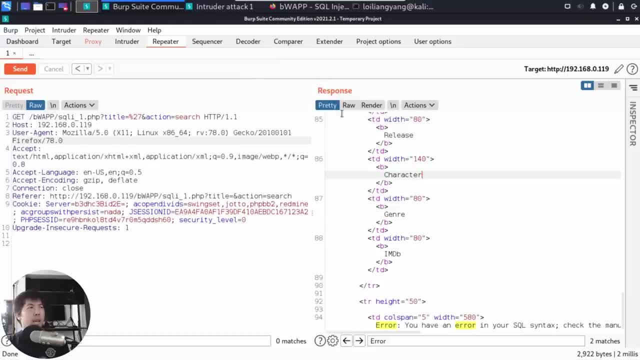 vulnerabilities inside an input field. all right, what we can do next is to deploy automation to also help us pull out all those usernames, password and look at all the different tables inside a database system. so what i can do now is go ahead and open up terminal. all right, so let 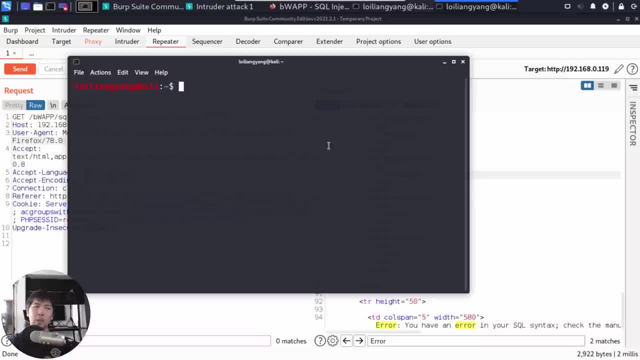 us zoom in a little more so that it is easier for you to see. so what i can do now is use sql map. so sql map is a structured query language that will actually do the injection automatically for us, and in this case, of course, we have identified the vulnerable field, so i can go ahead and enter. 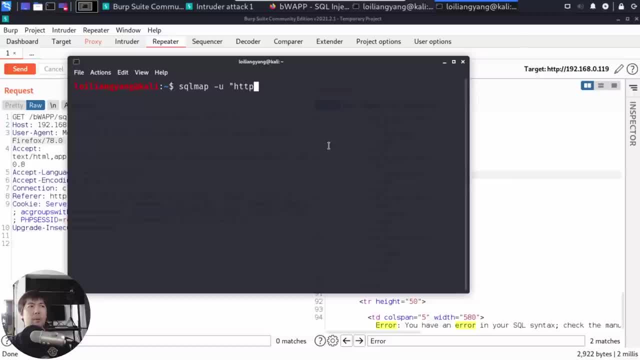 following, which is dash u for the url. in this case we have http, followed by colon double slash. all right, 192.168.0.119. and, of course, in the real world, as i've shared several times, you'll be going after a domain name. okay, so we have b w a p p and, as you can see on the left side, we have 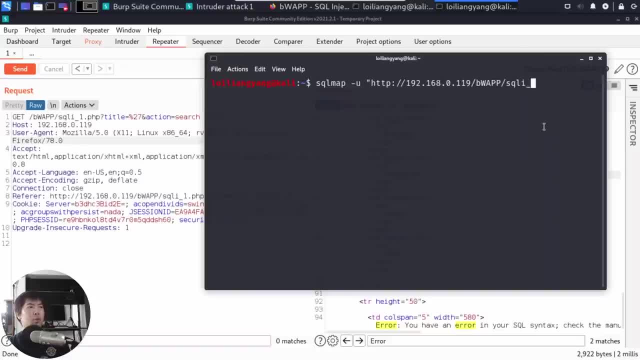 b, w, a, p, p slash sql. i underscore one dot php question mark title equal. okay, then we'll close it off with double quote. and now what we need to do is to actually specify the cookie, because we actually need to log into the site earlier in order to be able to gain access to look at all. 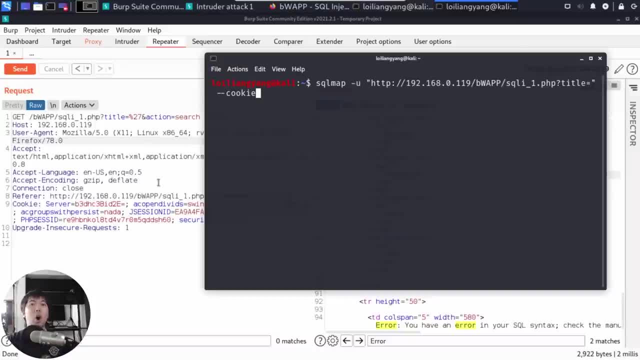 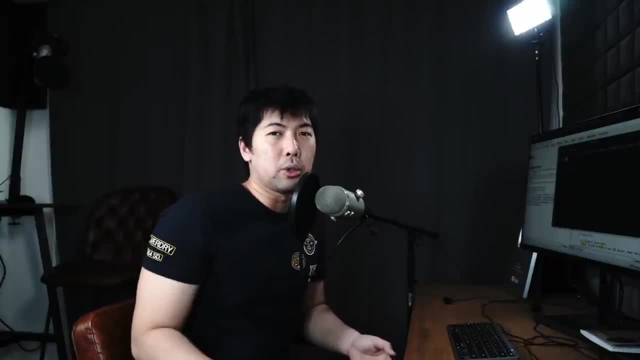 these functions and run all these different kind of ethical hacks and all these different kind of hacking techniques on a website or a server, so attacks don't just come from outside. that means unregistered users, unauthenticated users. attacks actually can come from inside, meaning that these are users who are registered inside your company, inside as a contractor, and they have access to. 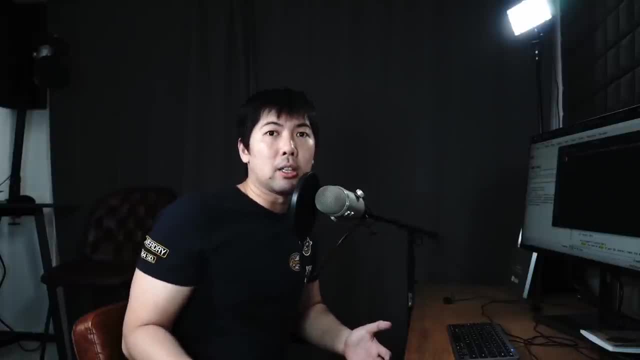 certain features and functions of a website and because they're authenticated, there's tend to be a zone of trust that is being provided or enabled for all these users so that they can run more elevated privileges or accesses to more elevated functions, which could then actually provide them access or indirect access to different parts of a. 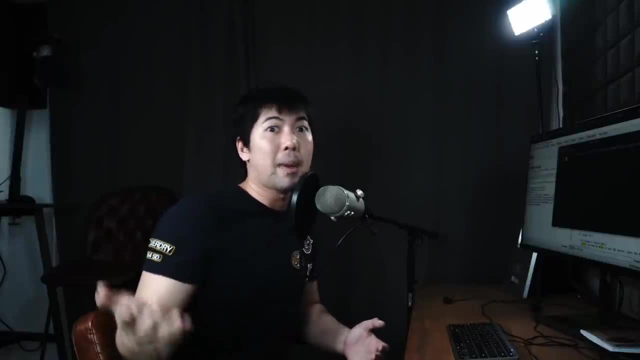 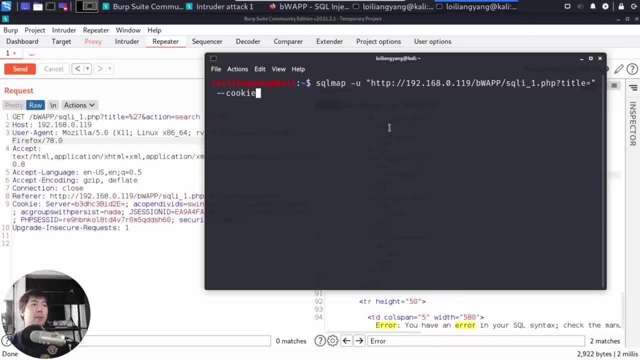 application system like a database table, all right, like a username, and pass a few credit card information because they're coming in with elevated privileges. so now, going back into the tutorial, i can do a double dash cookie equal. and now all i got to do is copy the. 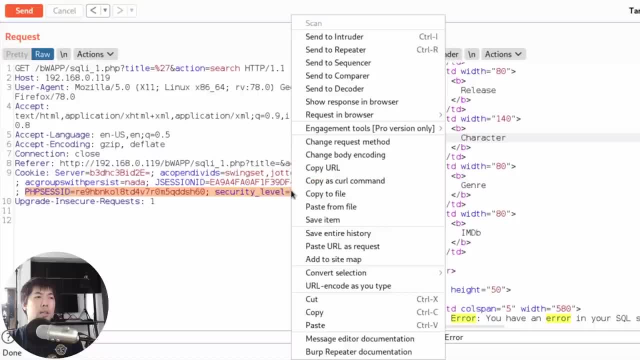 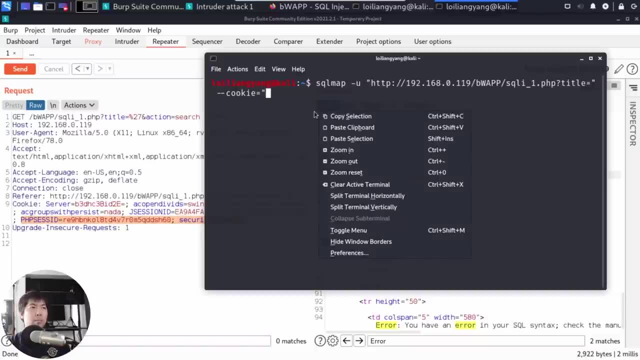 cookie: php session id over here. all right, so let's go ahead and do a copy. right click copy and go back to terminal and paste it over here. okay, so let's go ahead and do a double code: paste the selection. all right, so we have paste the selection right here at the end and go. 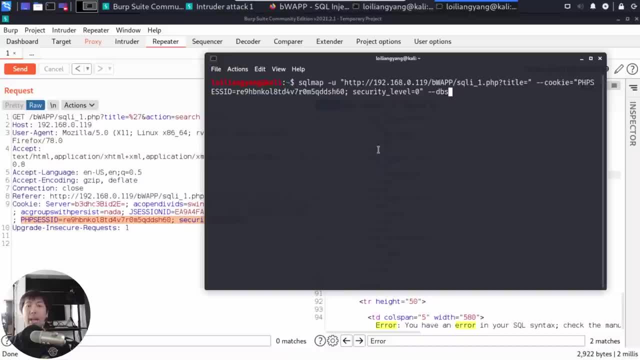 ahead and put a double quote to close it off. so what we're doing here is we have sql map dash u, and now we're going after this particular ip address or a domain name in the real world and we're testing out sql i. all right, underscore one dot php question mark title equal and we'll. 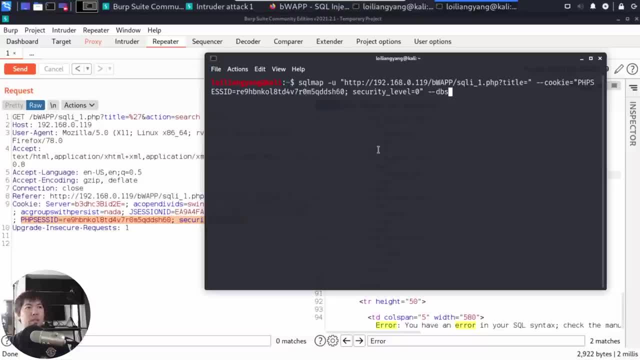 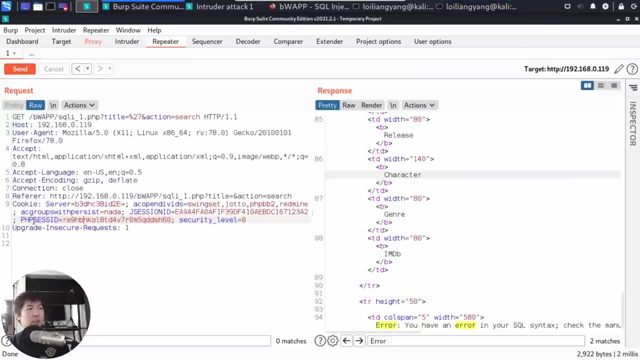 automatically fill it with sql map and followed by the cookie. all right, php session id as well. security level equals zero, all right, and double dash dbs so that we can pull out the database of information and, as you see here, all right, we have cookie information and because we need to log into, 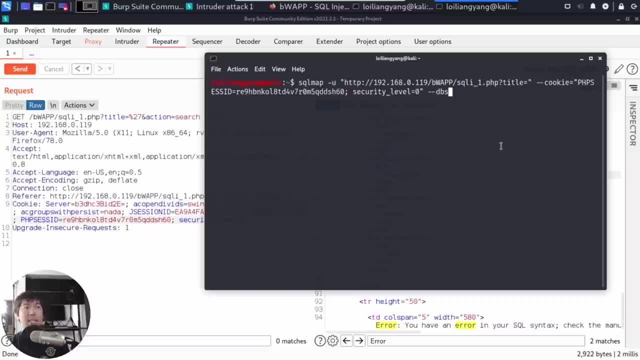 the site earlier, which is why we issue a php session id in order to gain access to different kind of features and functions inside the website. and now what we'll do? in three, two, one, we'll launch the attack and that's it game over. we are in and, in fact, what i can do now is launch a fresh query. 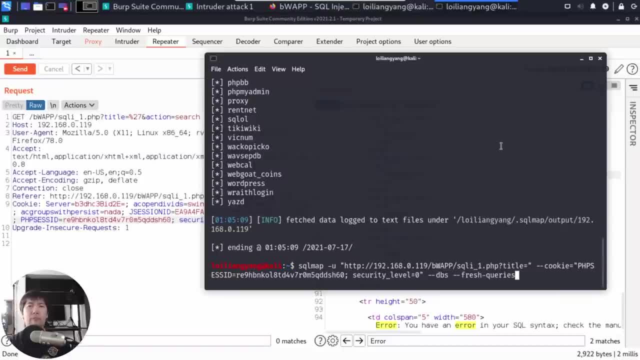 because earlier i was doing all this testing of the hacking techniques for you. so now let's do a fresh queries hit enter on this so we're re-injecting it and very quickly we're able to go to the website and we're able to launch the attack and that's it game over. we are in and in. 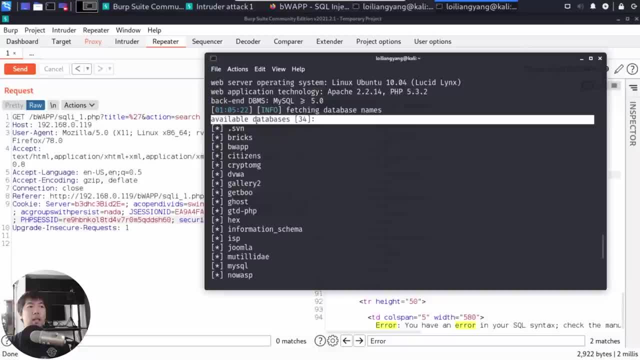 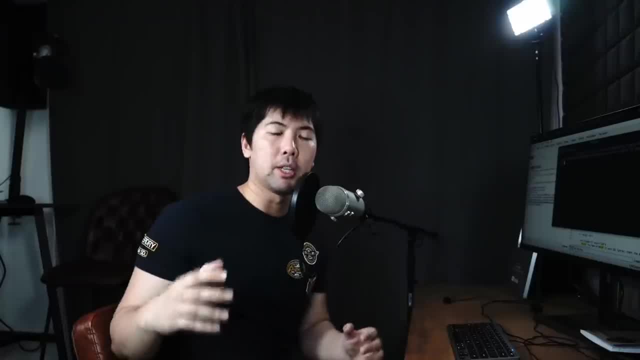 and we're able to launch the attack and that's it game over. we are in and in and we're able to gain access into the entire site. so right here we can see the available databases. so we have bricks, bwapp with citizens creep omg, all right. so what's happening is that you have the database. 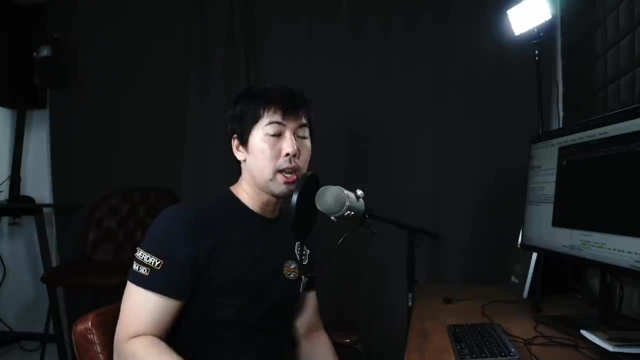 structure, all right, and followed by multiple tables inside the database, and all these tables will then have your rows and columns, kind of like an excel sheet where you use to pull out and store all this different kind of information, and we can change it directly from there and, of course, the 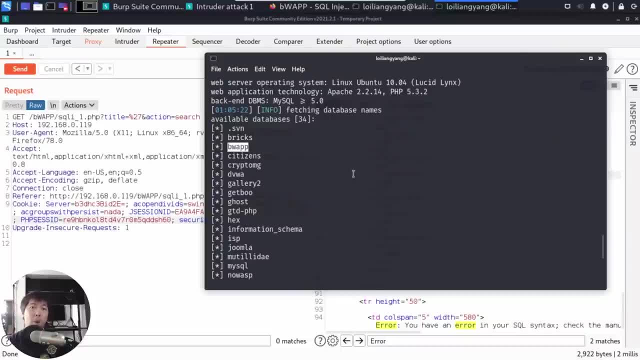 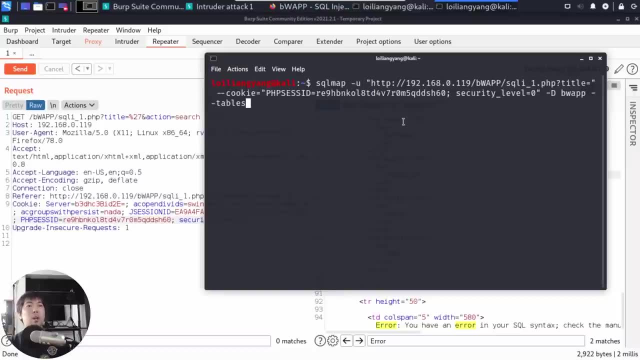 one that we're gunning for in today's case is bwapp, so let's go ahead and target this database. so, right here we have sql map, dash u for the url, all right, and then we have dash d, which is a database name that we're going after, followed by double dash tables to look for all those tables. 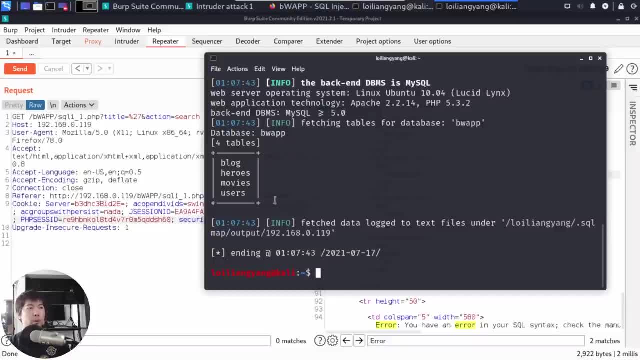 inside the database. so let's go ahead and run that. and right here we got the following results: four tables are being exposed. we have blog heroes, movies and users- okay, so i'm really, really interested in the users feed. so now what we do? we have modified the statement by using dash t. 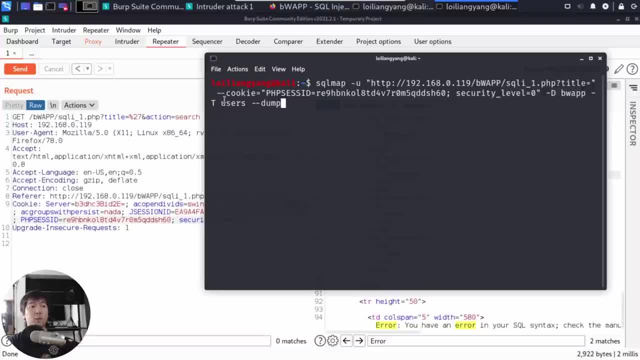 to specify the table name, followed by double dash, dom. so we are trying to dump out all of the usernames and passwords inside the database and inside the table. let's go ahead and hit enter on this, and it states the following: do you want to store hashes to a temporary file? 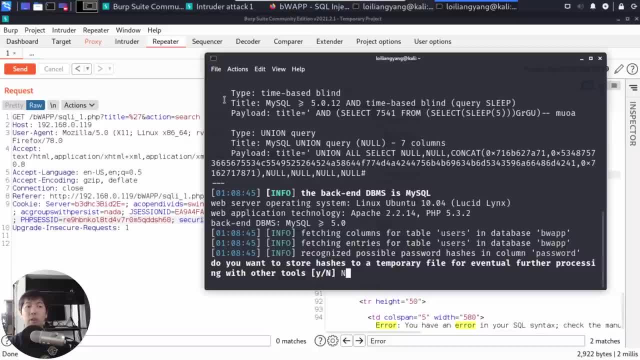 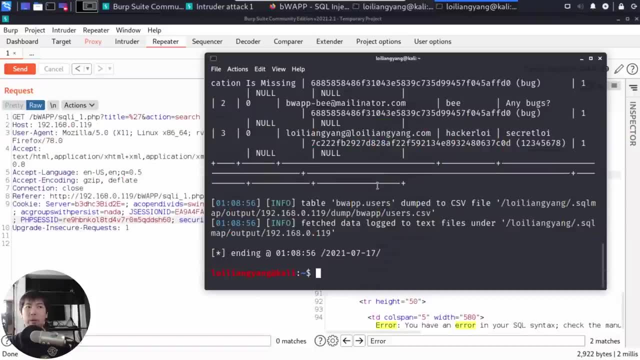 for eventual further processing with other tools. all right, let's enter no for that. you want to crack them via dictionary based attack? absolutely yes, and that's it game over. we are in and you can see right here. we got the following. all right, we have the email addresses, okay, as well as the. 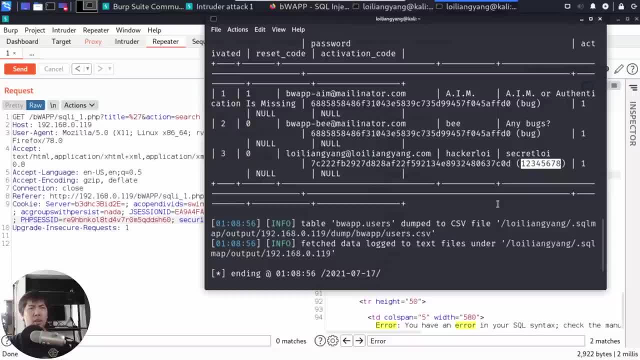 hashed value and the cracked value of those hashes. as you can see, right here we have a user called loylangyang, at loylangyangcom, followed by the password field: one, two, three, four, five, six, seven, eight. oh, that is really scary and pretty easy to do, which is frightening and you. 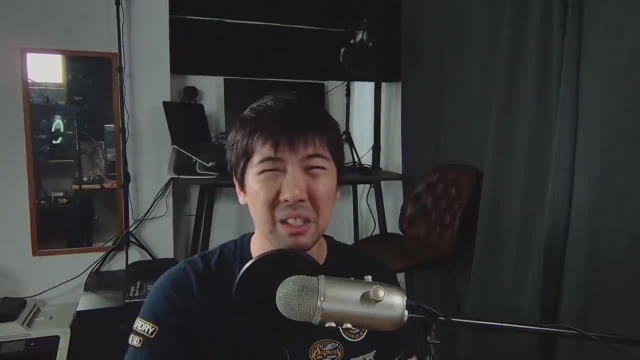 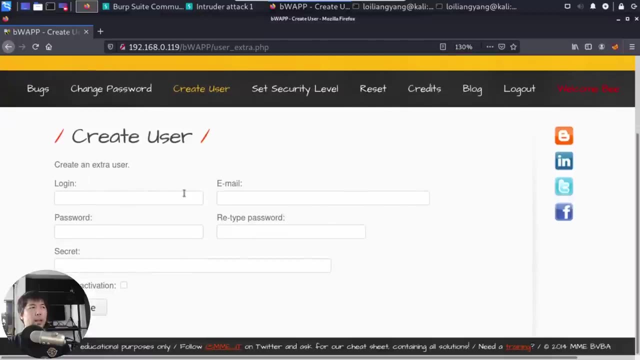 have to store strong, secure passwords, else your accounts can be hacked easily in any databases on any websites. so what i will do next now is go ahead and click create user. all right, so we're back to the website. i want to create a user and let you see. all right, what password are we setting? 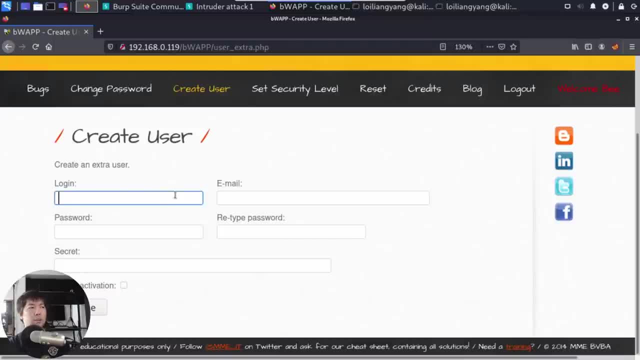 so now i will enter the following login information: okay, so i can enter mr hackerloy. okay, an email address. i'm going to put it as loylangyang at loylangyangcom. all right, and password view. so now you have no idea what is the password. okay, so we'll do a. 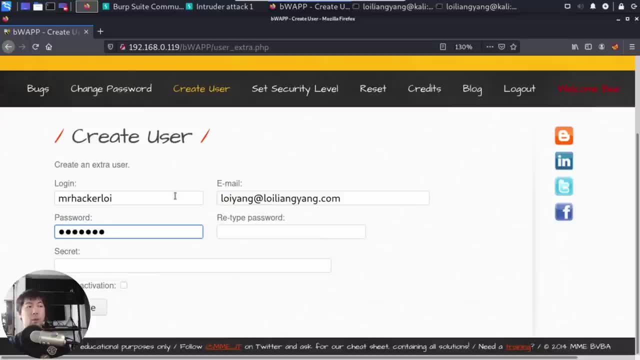 password cracking into this account and i'll enter the password view. all right, so you have no idea what is the password now, okay, and we'll try to crack it using the same tool that we used earlier and secret- i'll say secret loy. okay, so now let us go ahead and click create user and you can see. 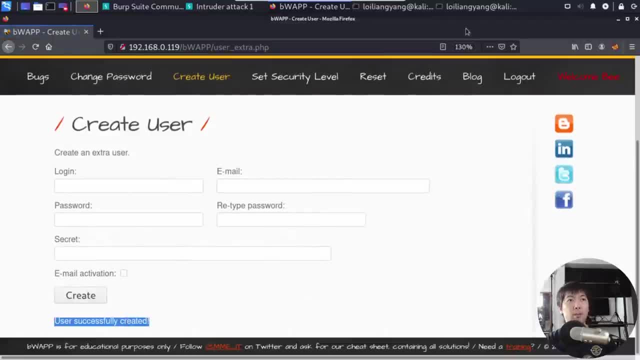 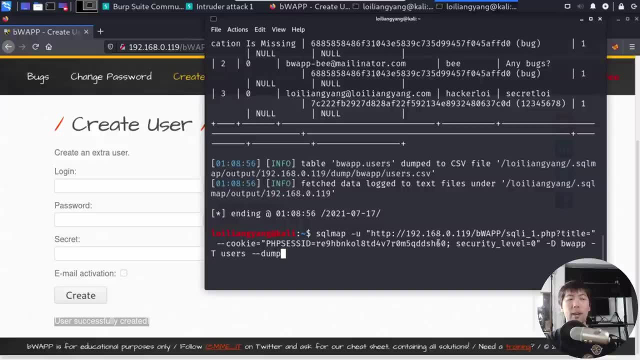 right at the bottom user successfully created. all right, so now, if we go back into our sql map tool right here, what i can do now is go ahead and do a same query, okay, and if you hit enter on this, you want to store hashes to temporary file for eventual further processing. so let's enter no for that. so